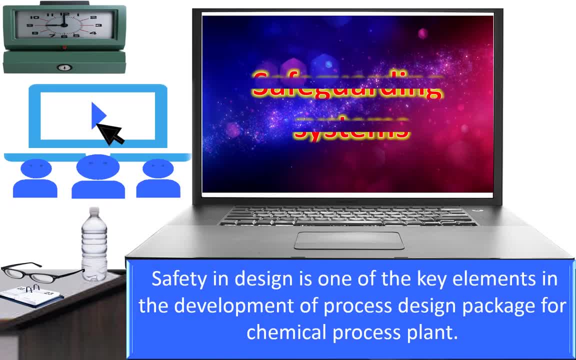 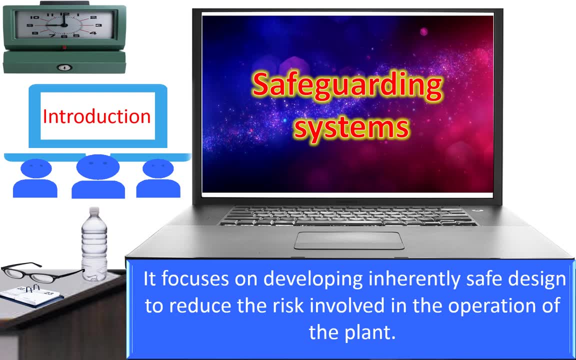 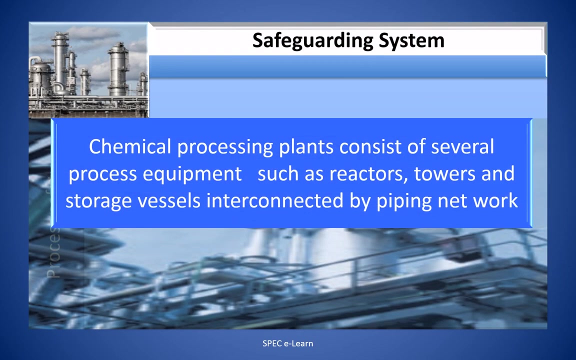 Safeguarding Systems. Safety in design is one of the key elements in the development of process design package for chemical process plant. It focuses on developing inherently safe design to reduce the risk involved in the operation of the plant. Process plants consists of several process equipment, such as: 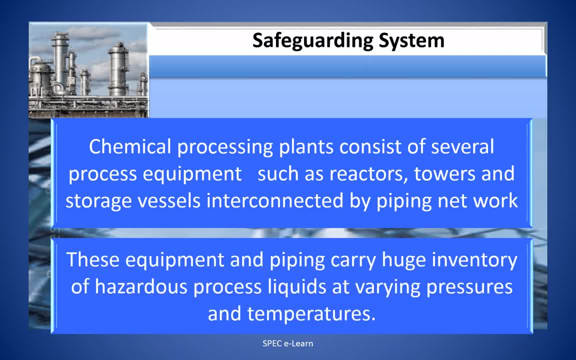 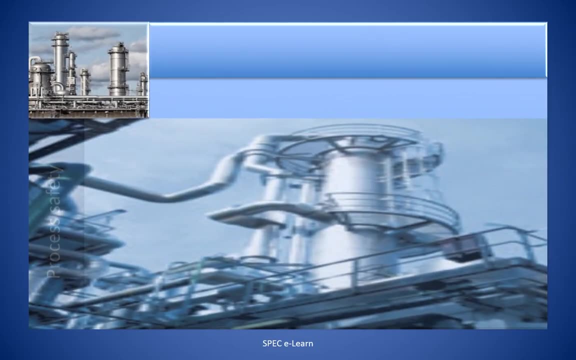 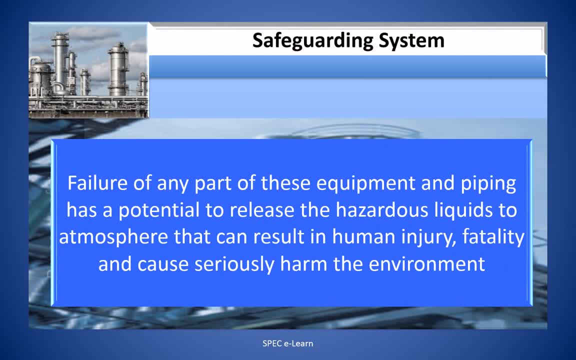 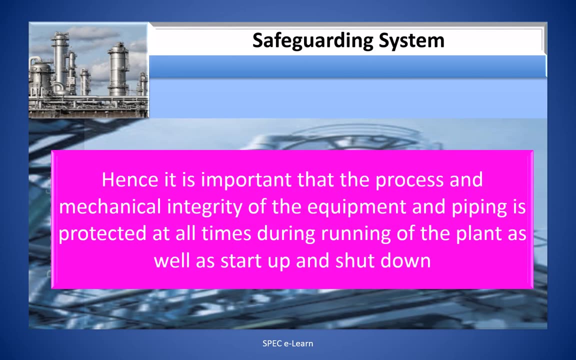 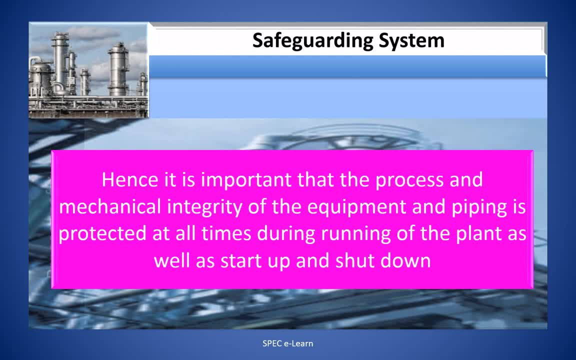 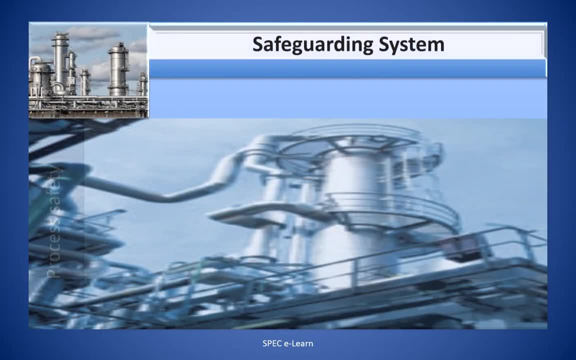 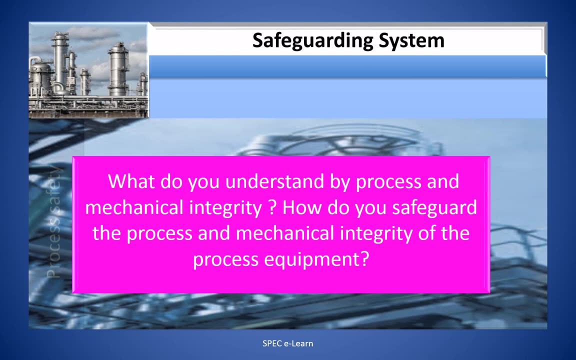 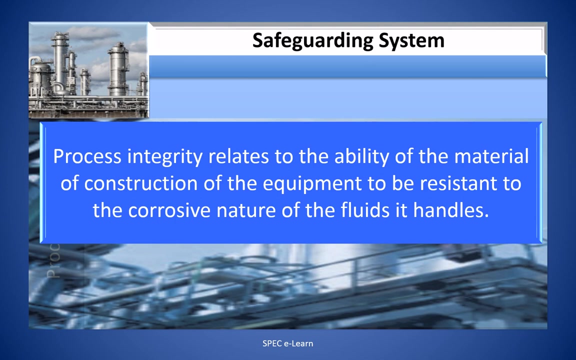 and piping is protected at all times during running of the plant, as well as startup and shutdown. What do you understand by process and mechanical integrity? How do you safeguard the process and mechanical integrity of the process equipment? Process integrity relates to the ability of the material, of construction of the equipment. 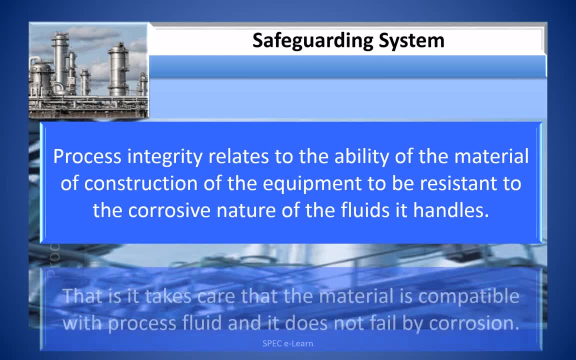 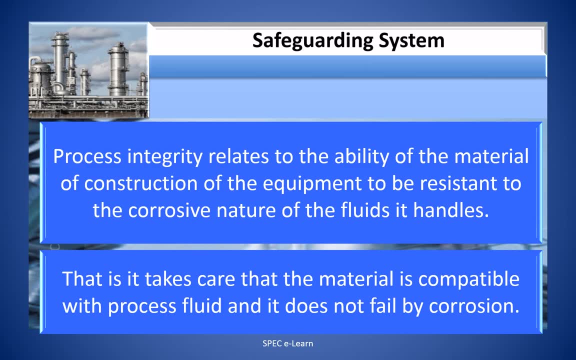 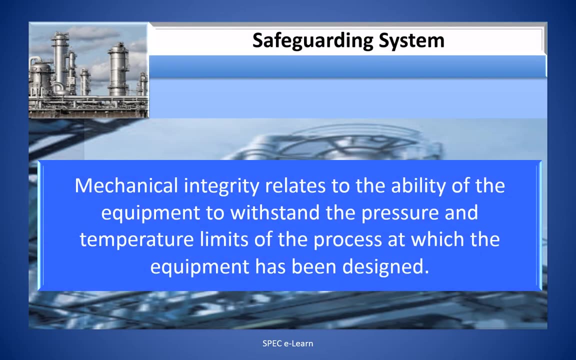 to resist the corrosive nature of the fluid it handles. That is, it takes care that the material is compatible with process fluid and it does not fail by corrosion. Mechanical integrity relates to the ability of the equipment to withstand the pressure and temperature limits of the process at which 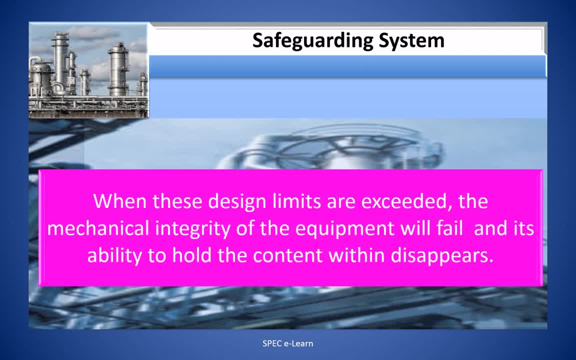 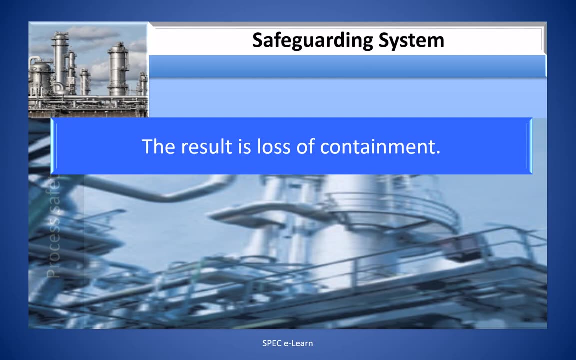 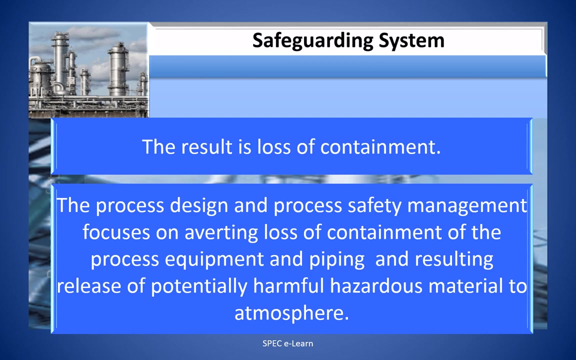 the equipment has been designed. When these design limits are exceeded, the mechanical integrity of the equipment will fail and its ability to hold the content within disappears. The result is loss of containment. The process design and process safety management focuses on averting loss of containment of process equipment and piping and resulting 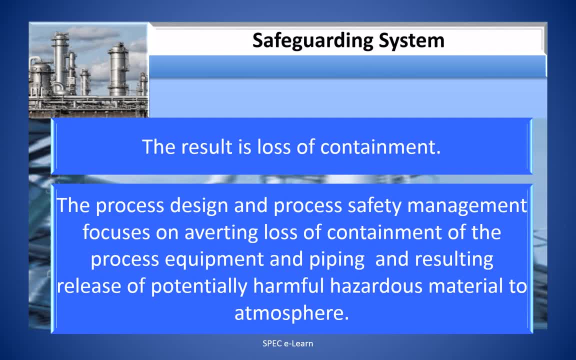 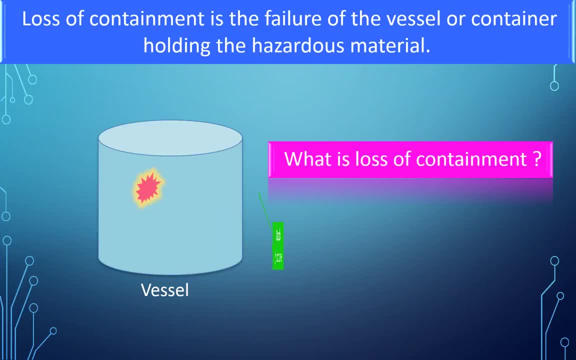 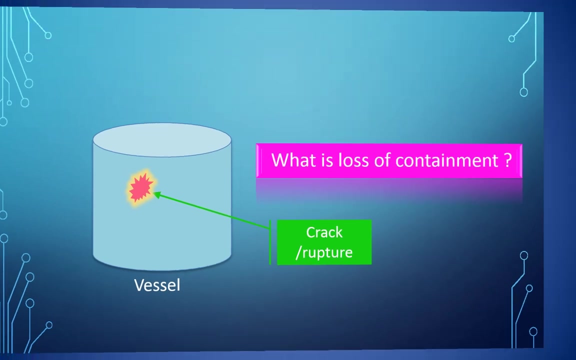 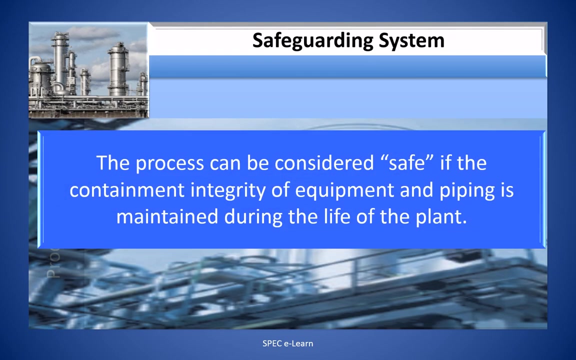 release of potentially harmful hazardous material to atmosphere. What is loss of containment? Loss of containment is the failure of the vessel or the container holding the hazardous material. It may be a crack on or rupture of the vessel wall, as shown in the figure. The process can be considered safe if the containment integrity of equipment and piping 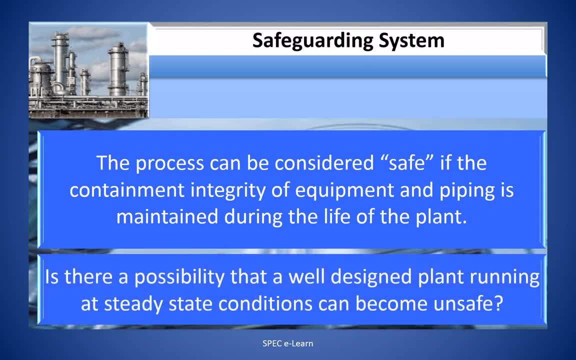 is maintained. The process can be considered safe if the containment integrity of equipment and piping is maintained during the life of the plant. The process can be considered safe if the containment integrity of equipment and piping is maintained during the life of the plant. Is there a possibility that a well-designed plant? 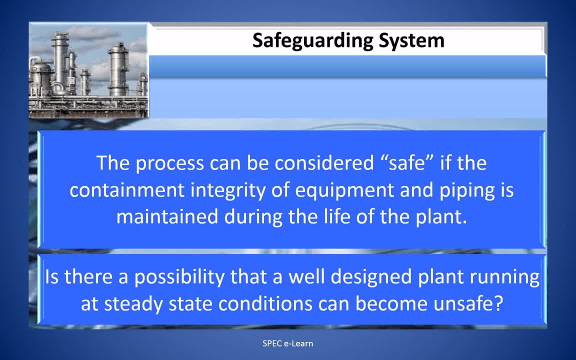 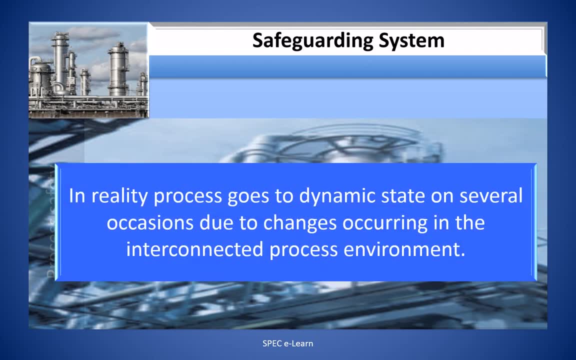 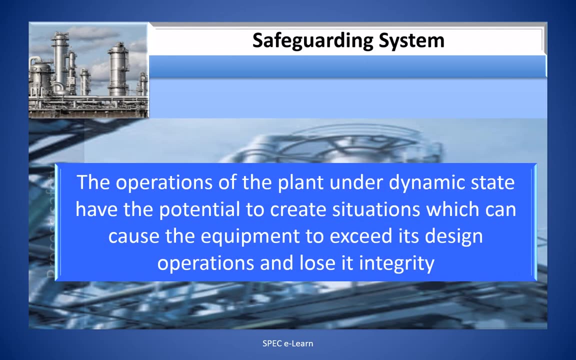 running at steady-state conditions can become unsafe. In reality, process goes to dynamic state on several occasions due to changes occurring in the interconnected process environment. The operations of the plant have the potential to create situations which can cause the equipment to exceed its design operating parameters and lose its integrity. 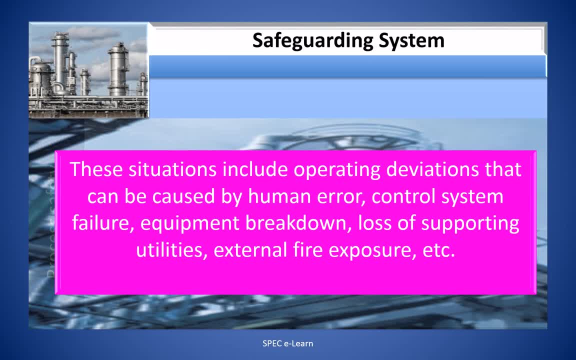 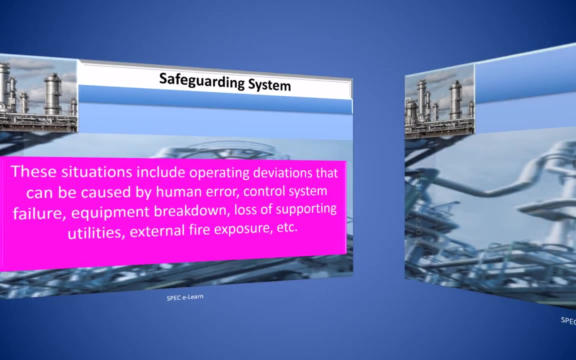 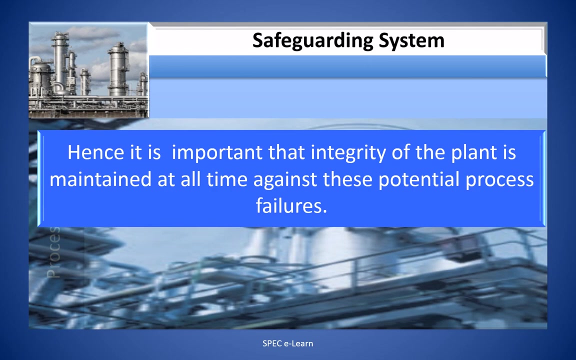 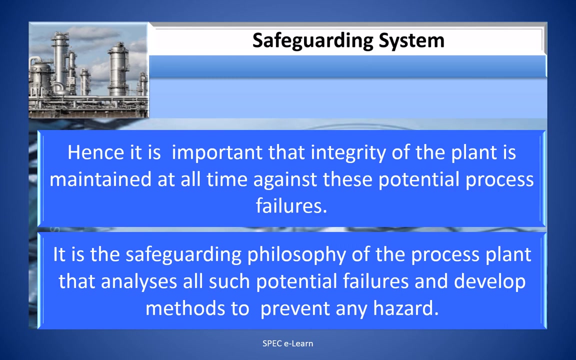 These situations include operating deviations that can be caused by human error, control system failure, equipment breakdown, loss of supporting utilities, external fire exposure, etc. Hence, it is important that the integrity of the plant is maintained at all times. Case trailing The mobilization andiod Freeman University. 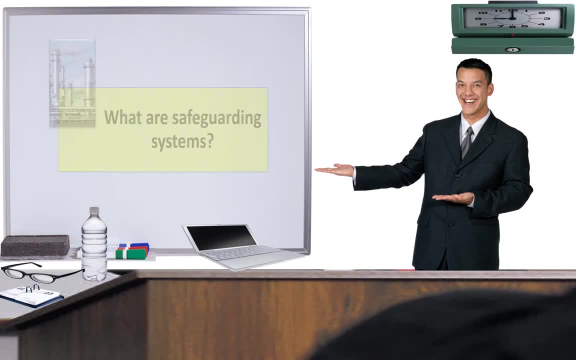 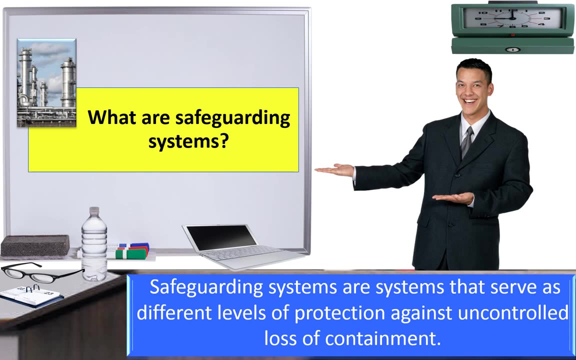 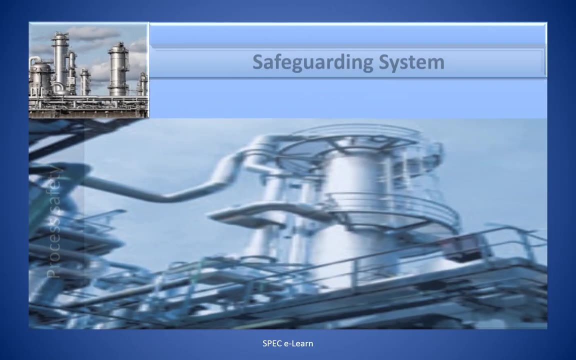 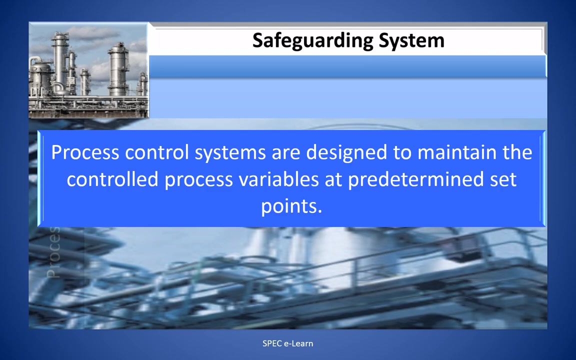 It is a safeguarding philosophy of the process plant that analyzes all such potential failures and develops methods to prevent any hazard. What are safeguarding systems? Safe Guarding Systems are systems that serve as different levels of protection against uncontrolled loss of containment. Process control systems are designed to maintain the controlled process variable at predetermined set points. 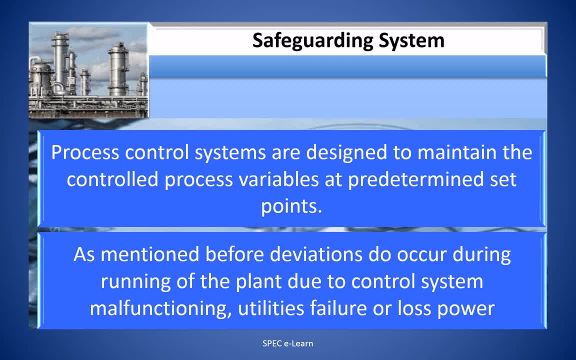 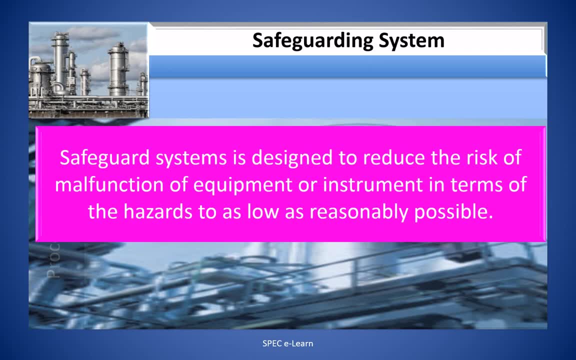 As mentioned before, deviations do occur during the running of the plant due to control system, malfunctioning utilities, failure or loss of power. Safeguard systems are designed to reduce the risk of malfunction of the equipment or instrument, in terms of the hazards, to as low as reasonably possible. 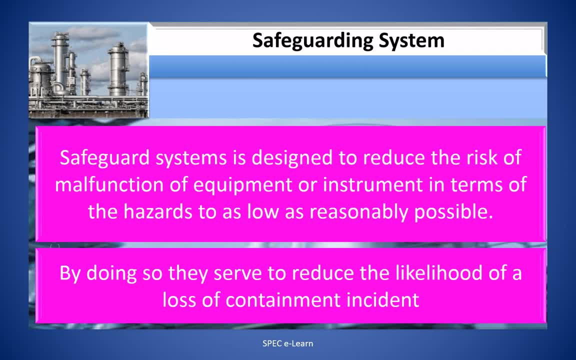 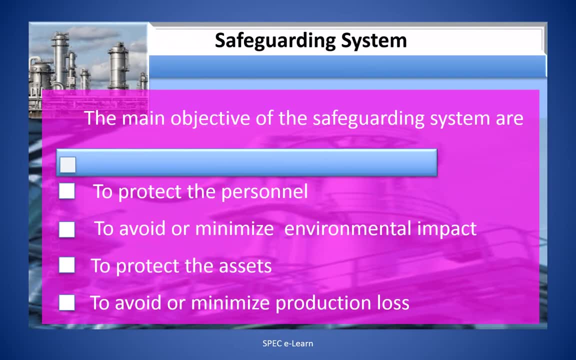 By doing so, they serve to reduce the likelihood of a loss of containment incident. The main objective of the safeguarding systems are: to protect the personnel. to avoid or minimize the environmental impact. to protect the assets. to avoid or minimize the protection loss. 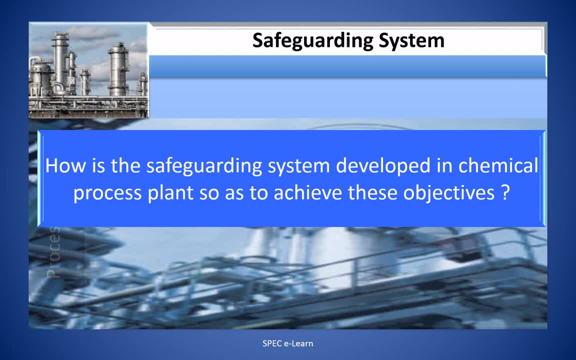 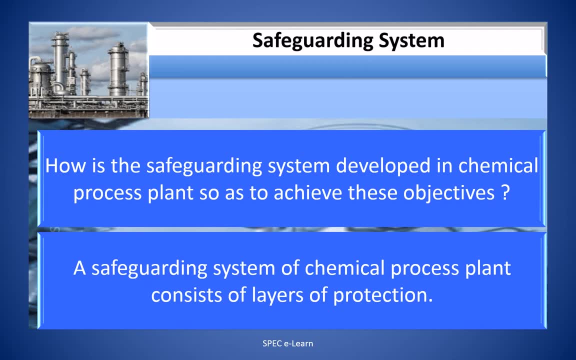 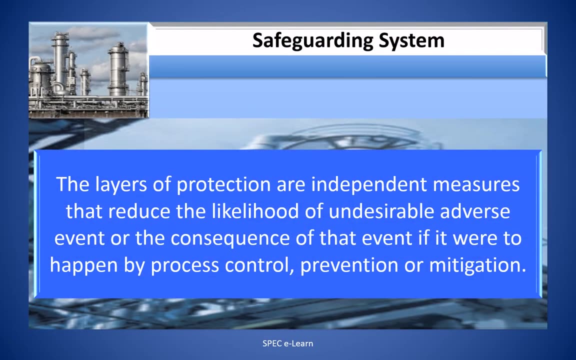 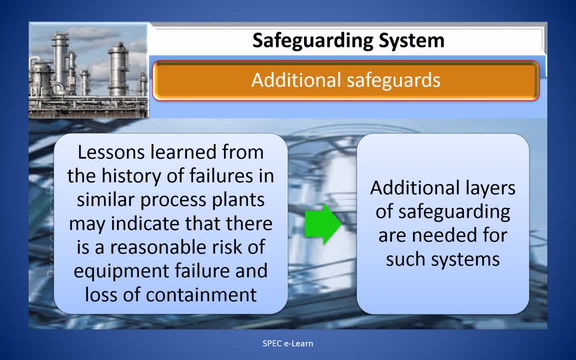 Every process equipment is subjected to detailed safety risk analysis and layers of protection are provided based on the findings. Additional safeguards: lessons learned from the history of failures in similar process plants may indicate that there is Additional safeguards: lessons learned from the history of failures in similar process plants may indicate that there is. 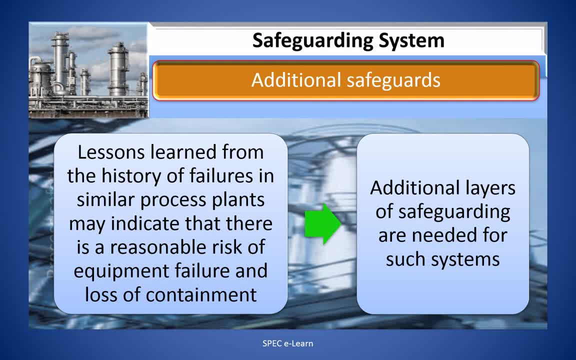 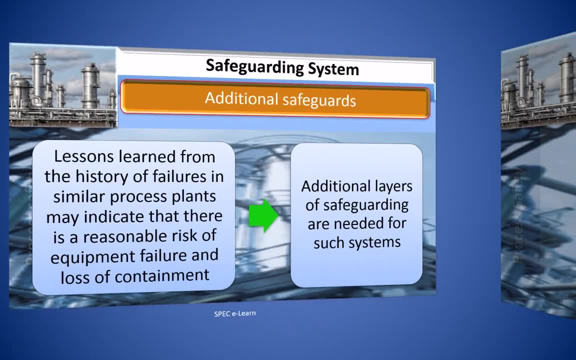 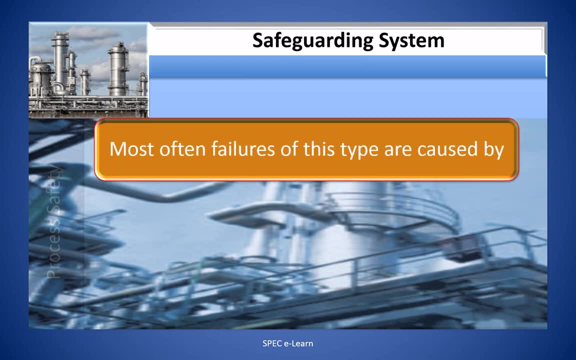 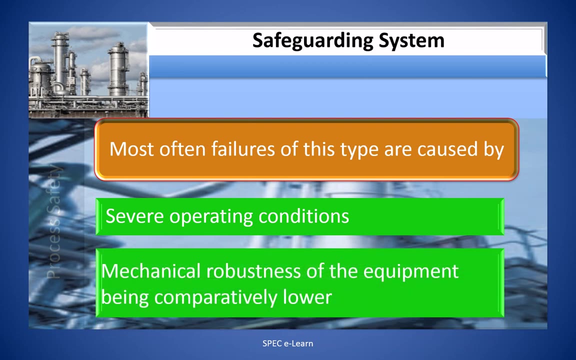 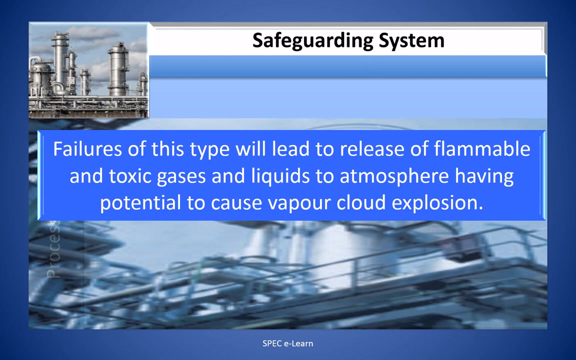 sufficient bound conditions for such systems. most often, failures of this type are caused by severe operating conditions, at mechanical robustness of the equipment being comparatively lower. Failures of this type will lead to release of flammable and toxic gases and liquids to atmosphere. 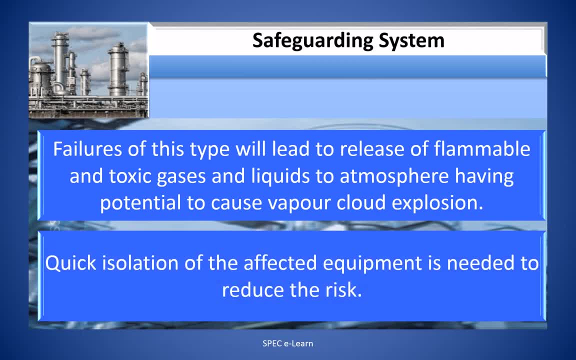 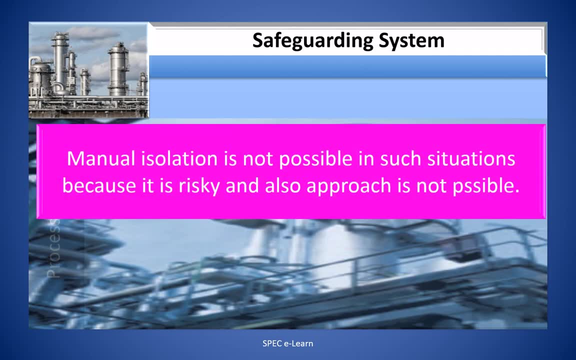 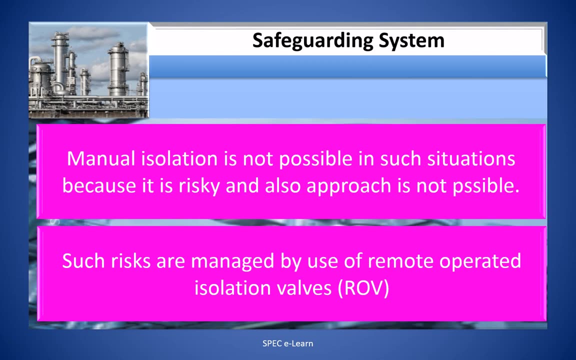 having potential to cause vapor cloud explosion. Quick isolation of the affected equipment is needed to reduce the risk. Manual isolation is not possible in such situations because it is risky and also approach is not possible. Such risks are managed by use of remote operated isolation valves. 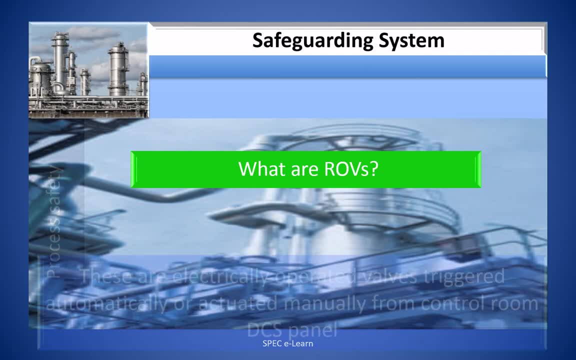 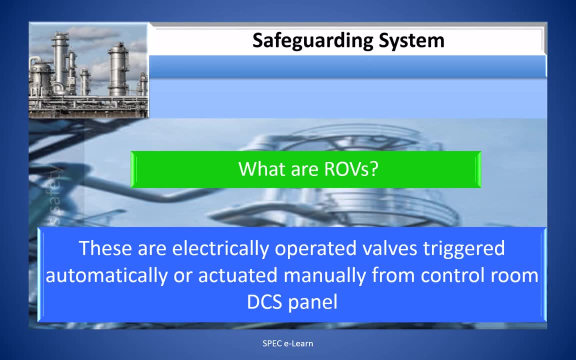 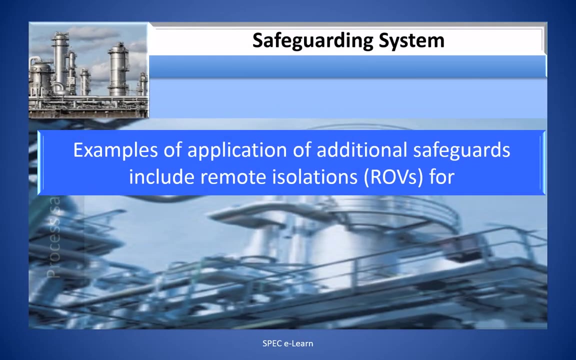 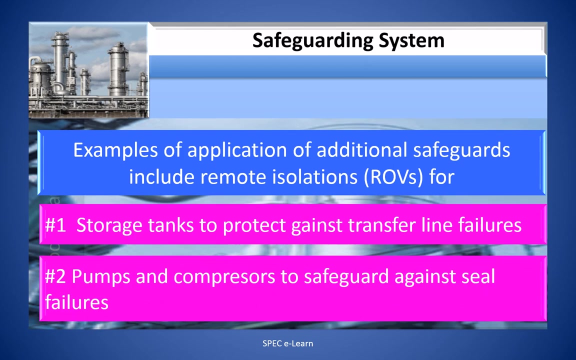 What are ROVs? These are electrically operated valves triggered automatically or actuated manually from control room DCS panel. Examples of application of additional safeguards include Remote isolation valves or ROVs for: 1. Storage tanks to protect against transfer line failures. 2. Pumps and compressors to safeguard against seal failures. 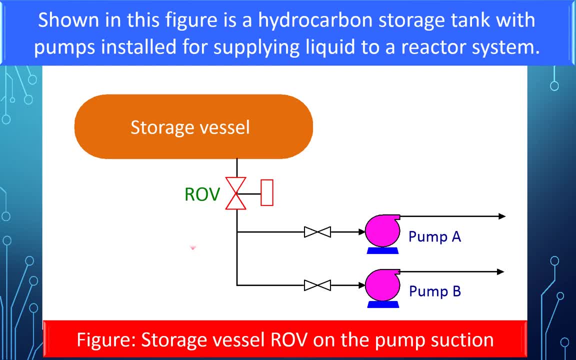 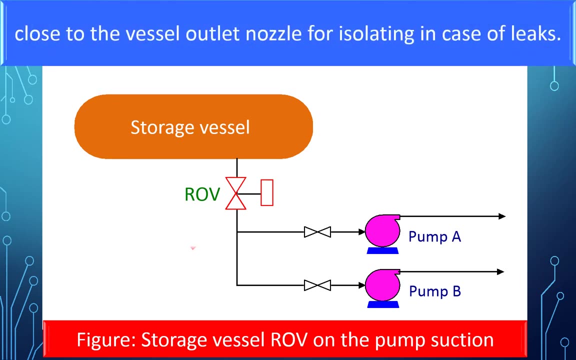 Shown in this figure is a hydrocarbon storage tank with pumps installed for supplying water. This tank has a huge inventory of flammable liquid. Note: this tank is provided with ROV at the pump suction line close to the vessel outlet nozzle for isolating in case of leaks. 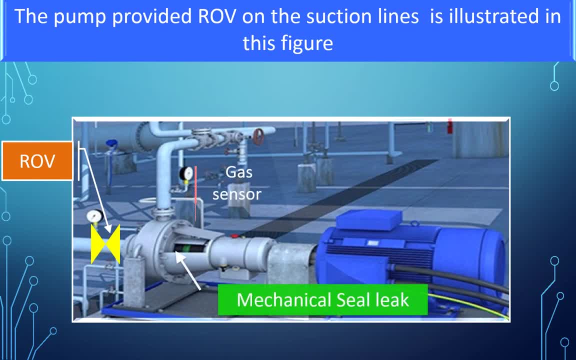 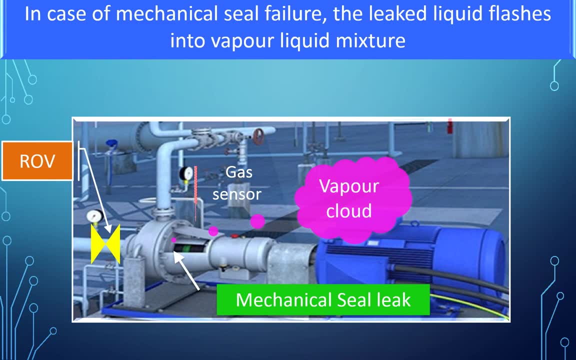 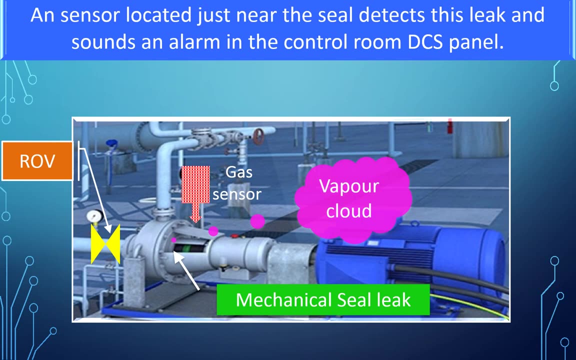 The pump provided with ROV on the suction line is illustrated in this figure. In case of mechanical seal failure, the leaked liquid flashes into vapor liquid mixer. A sensor located just near the seal detects this leak and sounds an alarm in the control room DCS panel. 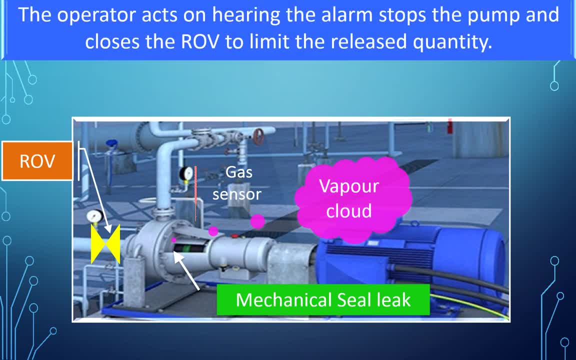 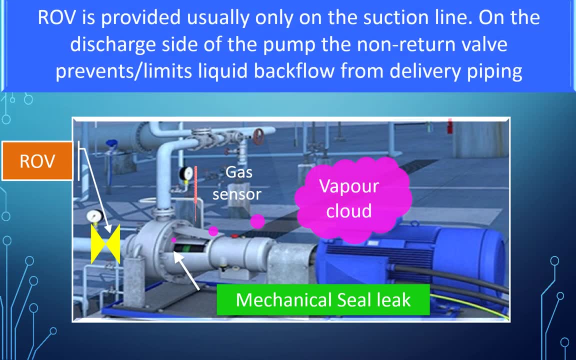 The operator acts on hearing the alarm, stops the pump and closes the ROV to limit the release quantity. ROV is provided usefully on the suction line. On the discharge side of the pump the non-return valve prevents or limits the liquid backflow from delivery piping. 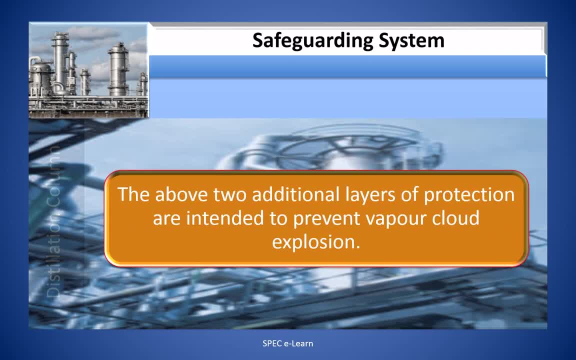 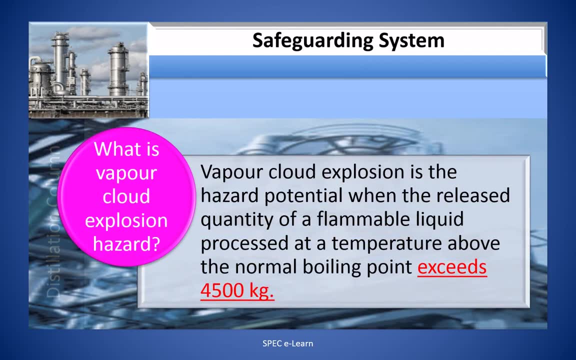 The above two additional layers of protection are intended to prevent vapor cloud explosion. Vapor cloud explosion is the hazard potential when the release quantity of flammable liquid processed at a temperature above the normal boiling point exceeds 4500 kg. This is the risk potential associated with vessel A. 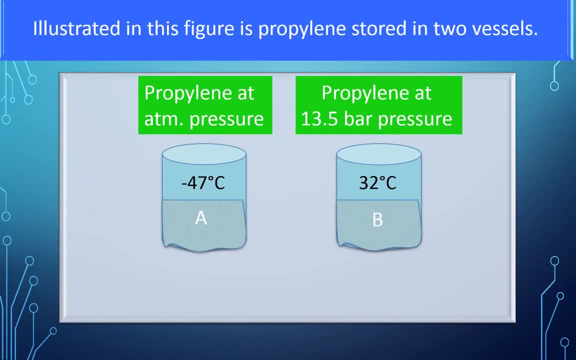 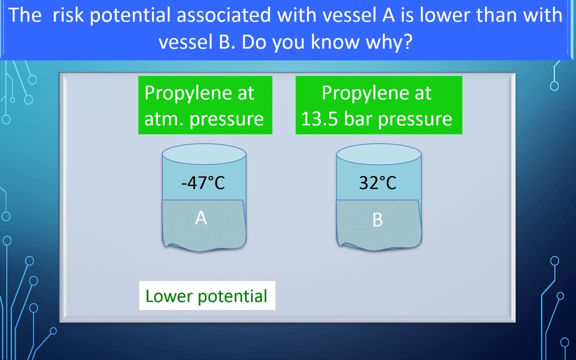 In less detailed in this figure is properly installed in two vessels: One vessel at atmospheric pressure at minus 47 degree centigrade, The other at 13.5 bar pressure at 32 degree centigrade. The risk potential associated with vessel A is slower than with vessel B. 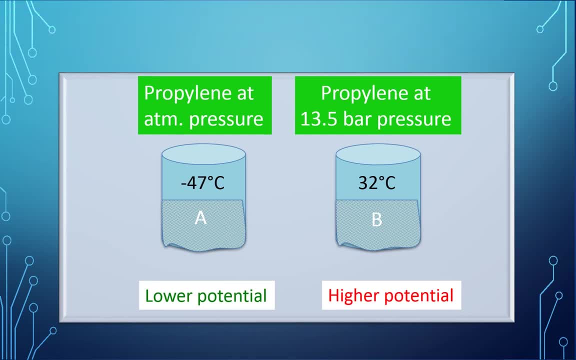 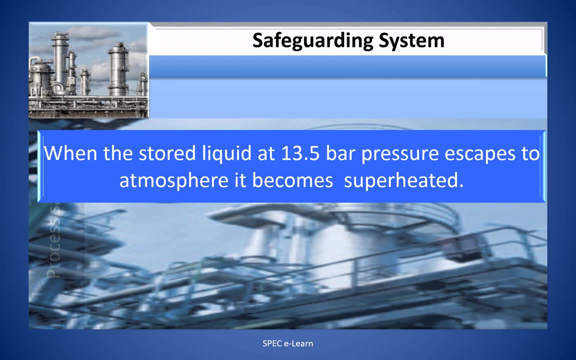 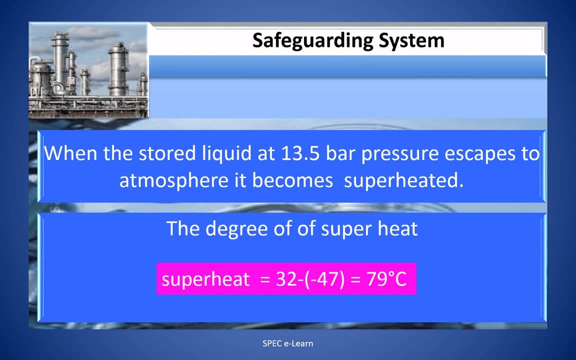 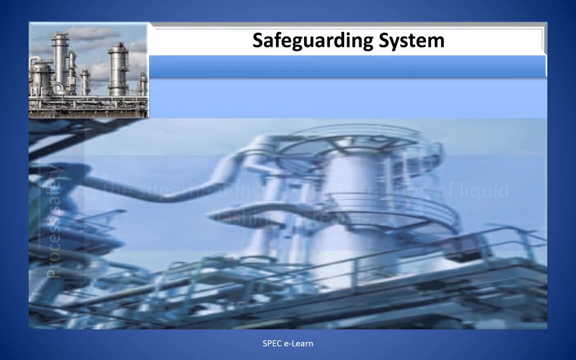 Do you know why? When the stored liquid at 13.5 bar pressure escapes to atmosphere, it becomes superheated. The degree of superheat equal to 32 minus minus 47 equal to 79 degree centigrade. As the superheat increases, the fraction of liquid flashing increases. 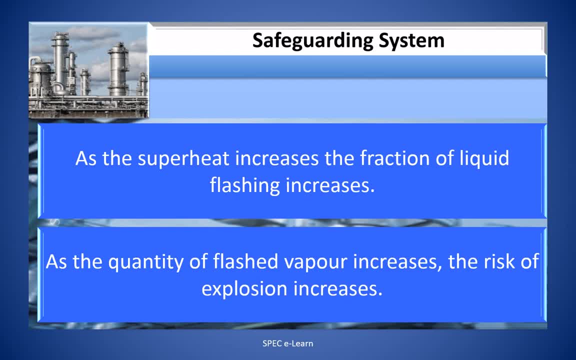 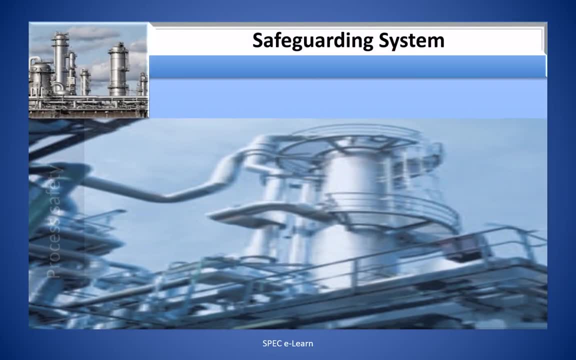 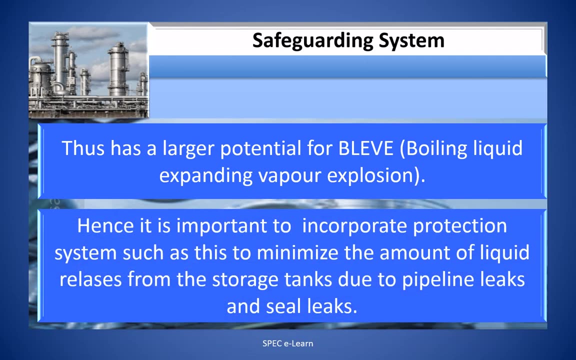 As the quantity of flashed vapor increases, the risk of explosion increases, Thus has a larger potential for BLEEV. Hence it is important to incorporate protection system such as this to minimize the amount of liquid release from the storage tanks due to pipeline leaks and sea leaks. 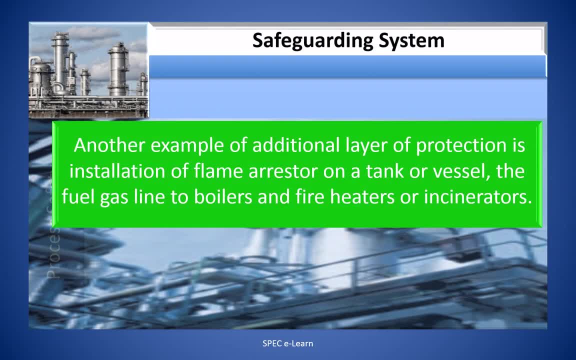 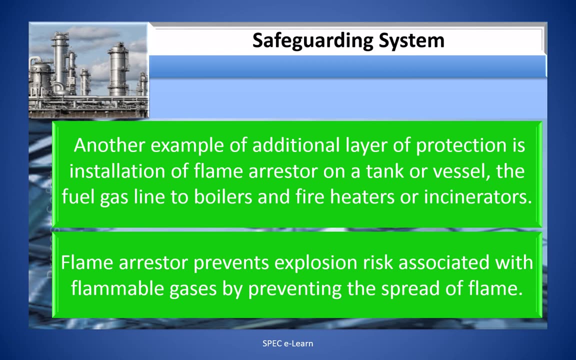 Another example of additional layer of protection is installation of flame arrester on a tank or a vessel, The flue gas line to boilers and fire heaters or incelerators. Flame arresters prevent explosion risk associated with flammable gases by preventing the spread of flame. 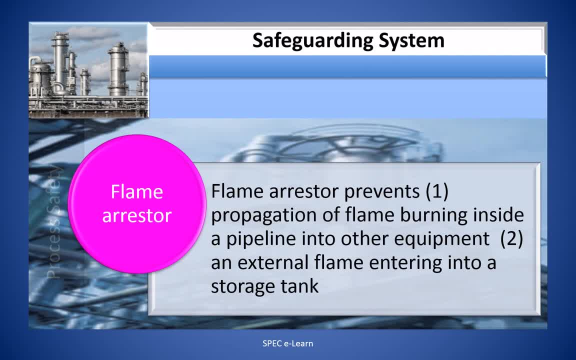 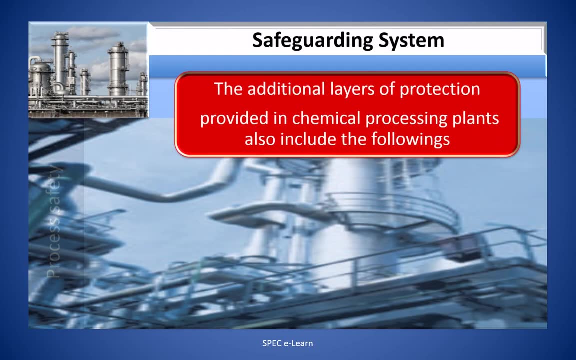 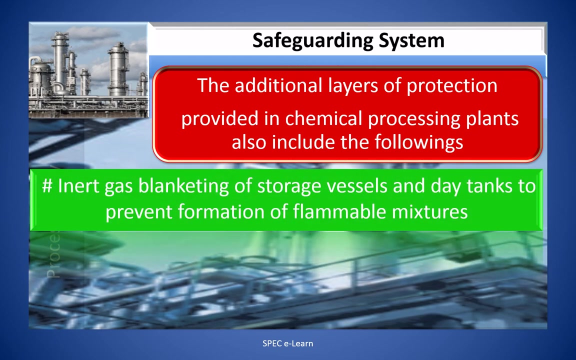 Flame arrester prevents: 1. Propagation of flame burning inside a pipeline into other equipment. 2. An external flame entering into a storage tank. The additional layers of protection provided in chemical processing plants also include the following: 1. Inert gas blanketing of storage vessels and day tanks to prevent formation of flammable mixes.